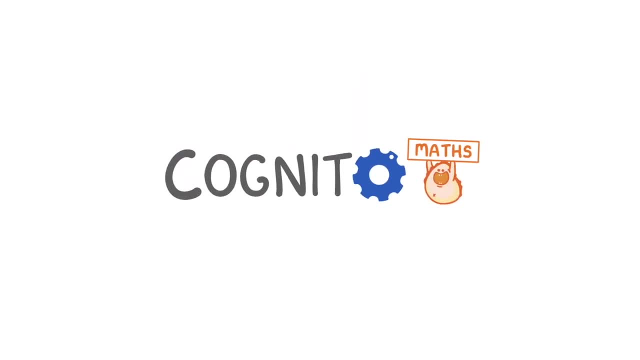 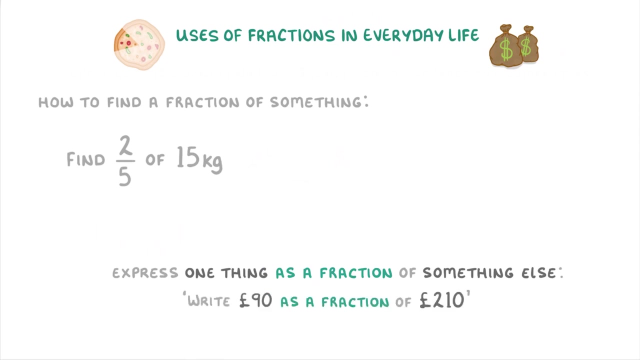 In this video we're looking at some of the uses of fractions in everyday life, So we'll cover how to find a fraction of something, like finding two fifths of 15 kilos, and how to express one thing as a fraction of something else, like writing 90 pounds as a fraction of 210 pounds. 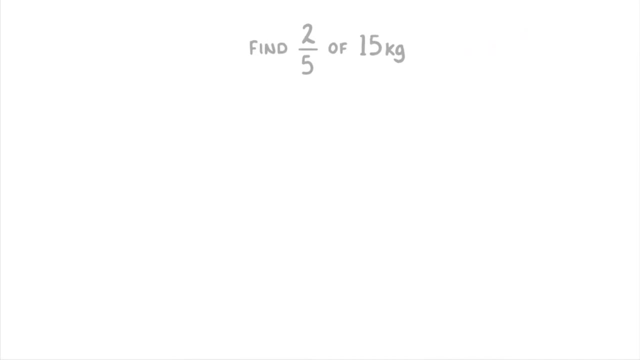 To find a fraction of something like two fifths of 15 kilos. we write the 15 kilos as a fraction, So turn it into 15 over 1, which we're allowed to do, because 15 divided by 1 is just 15.. So we 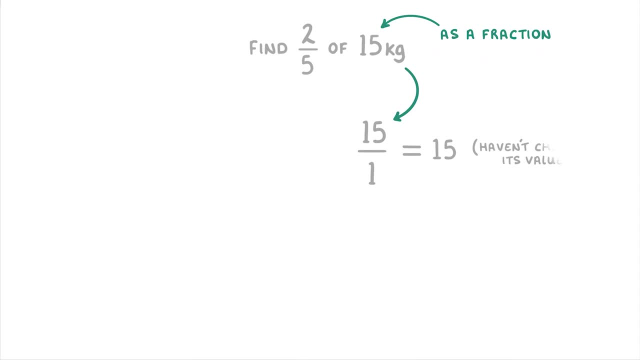 haven't actually changed its value at all. Next we have to multiply the two fractions together, So 2 over 5 times 15 is 15.. Next we have to multiply the two fractions together, So 2 over 5 times 15 is 15.. Next we have to multiply the two fractions together, So 2 over 5 times 15 is. 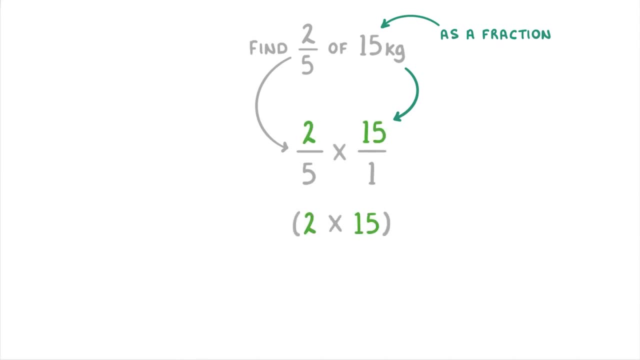 15 over 1,, which means 2 times 15, divided by 5 times 1, or 30 over 5,, which is 6.. So the answer is 6 kilos. Let's try another one. In this question we're trying to find three quarters. 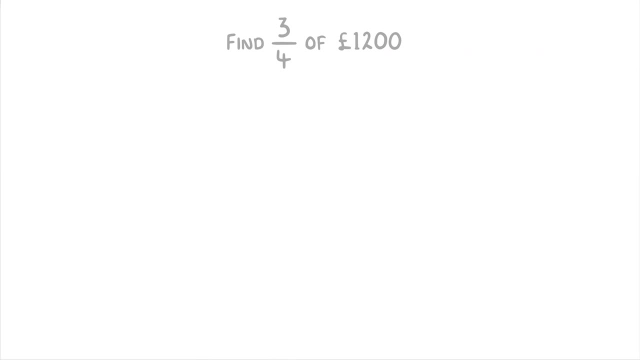 of 1,200 pounds. So the first thing we need to do is write an equation of three quarters of 1,200 times 1,200 over 1.. Then to multiply them, we do the 3 times 1,200 to get 3,600 as our 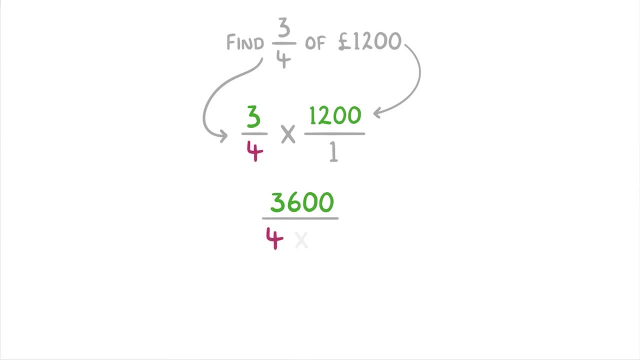 numerator and divide that by the 4 times 1 to get 4 as our denominator. So the answer is 3,600 over 4, which is just 900 pounds. Now to write one number as a fraction of another number, like 90 pounds as a fraction. 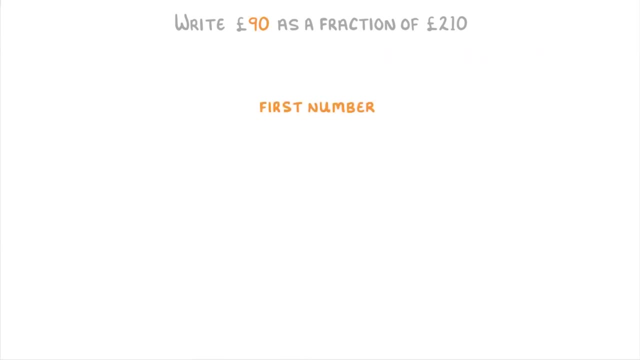 of 210 pounds. we just put the first number over the second number to make a fraction, And then we simplify the whole thing down as much as we can. So here we're, to do 90 over 210 and then simplify it by dividing top and bottom by 10: history 10.. 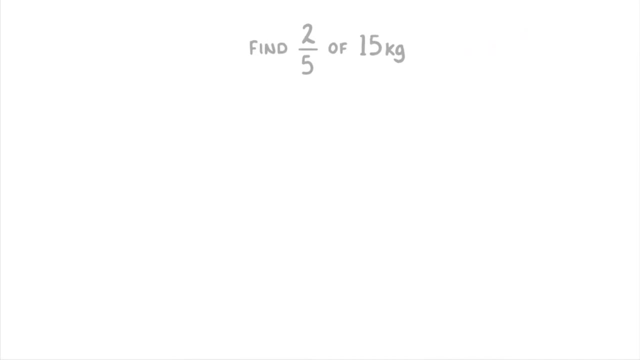 To find a fraction of something like two fifths of 15 kilos. we write the 15 kilos as a fraction, So turn it into 15 over 1, which we're allowed to do, because 15 divided by 1 is just 15.. So we 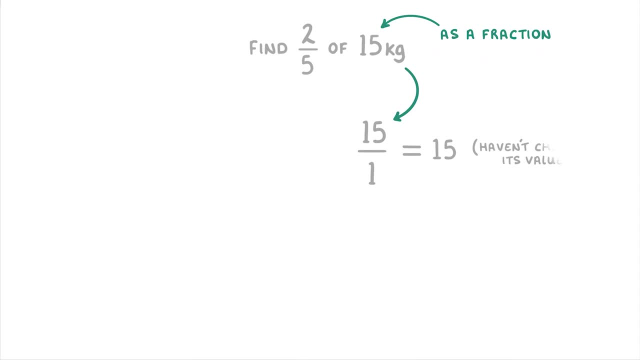 haven't actually changed its value at all. Next we have to multiply the two fractions together, So 2 over 5 times 15 is 15.. Next we have to multiply the two fractions together, So 2 over 5 times 15 is 15.. Next we have to multiply the two fractions together, So 2 over 5 times 15 is. 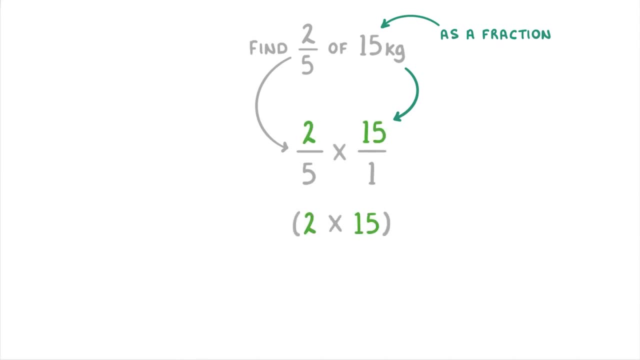 15 over 1,, which means 2 times 15, divided by 5 times 1, or 30 over 5,, which is 6.. So the answer is 6 kilos. Let's try another one. In this question we're trying to find three quarters. 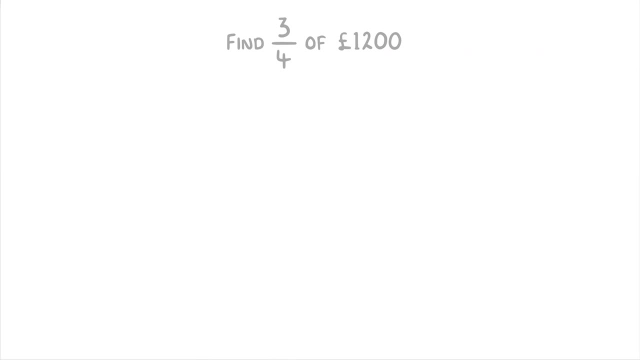 of 1,200 pounds. So the first thing we need to do is write an equation of three quarters of 1,200 times 1,200 over 1.. Then to multiply them, we do the 3 times 1,200 to get 3,600 as our 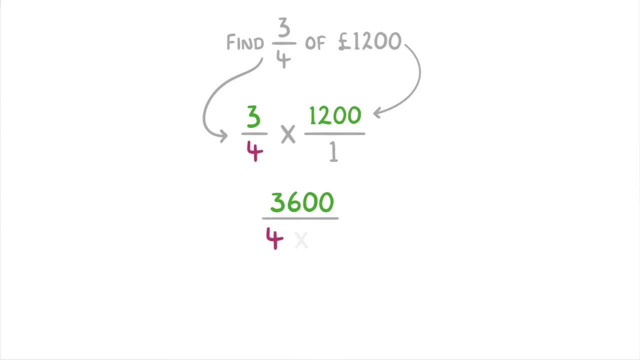 numerator and divide that by the 4 times 1 to get 4 as our denominator. So the answer is 3,600 over 4, which is just 900 pounds. Now to write one number as a fraction of another number, like 90 pounds as a fraction. 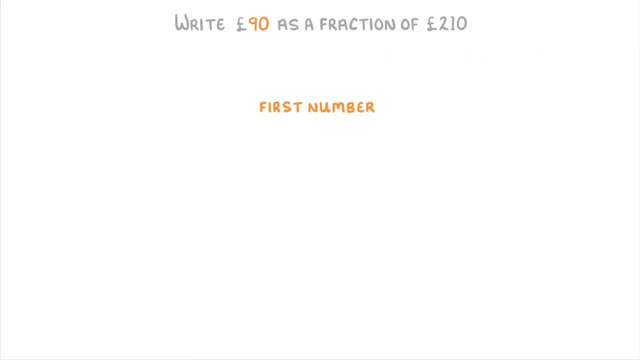 of 210 pounds. we just put the first number over the second number to make a fraction, and then we simplify the whole thing down as much as we can. So here we're, to do 90 over 210, and then simplify it by dividing the top and bottom. 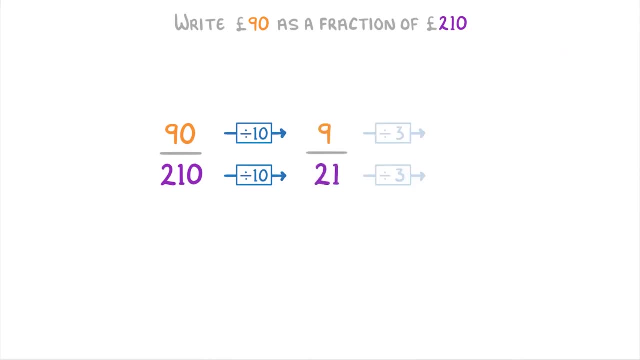 by 10 to get 9 over 21,, and then by 3 to get 3 over 7.. So 90 pounds is 3 sevenths of 210 pounds. In this next question we're asked to express 40 as a fraction of 16..